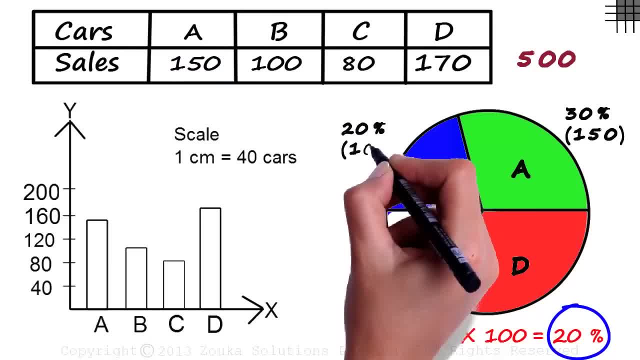 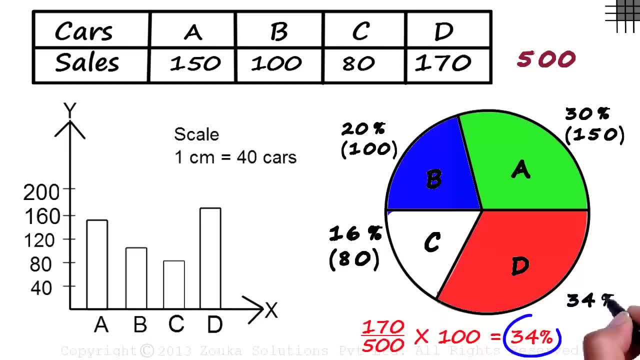 In the same way, B represents 20%, which is 100 cars, C represents 16%, which is 80 cars, And D represents 34%, that is, 170 cars. 150 is 30%, 50% of 500.. 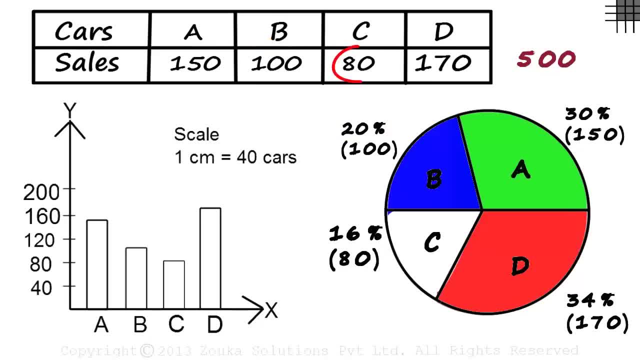 100 is 20% of 500.. 80 and 170 are 16 and 34% respectively. The region A covers 30% of the entire circle, Region B covers 20% of the entire circle, And region C and D represent 16 and 34% of the entire circle. 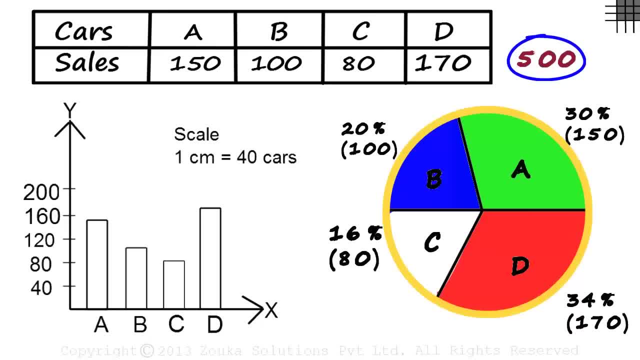 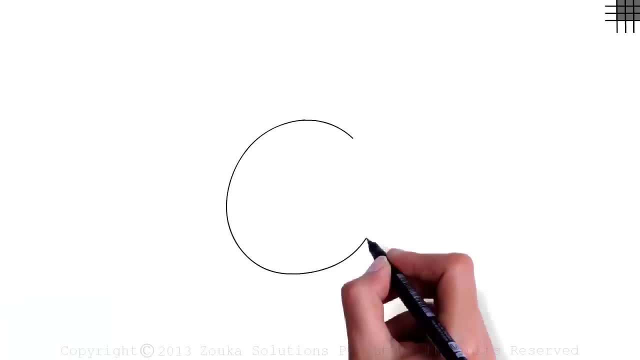 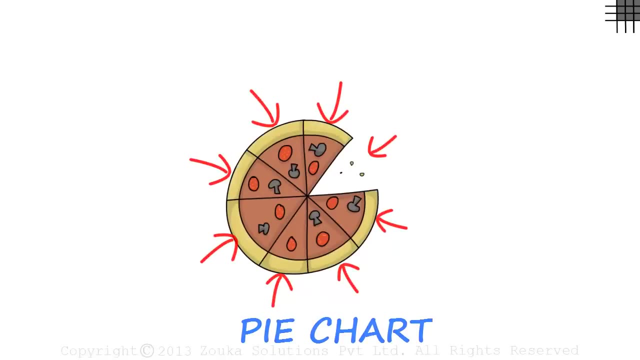 We use a circle to represent the total and make parts of it to represent each category. This type of representation is called a pie chart. And what's the best example of a pie chart? Yes, it's a pizza. It's a pie chart with equal parts or sectors. 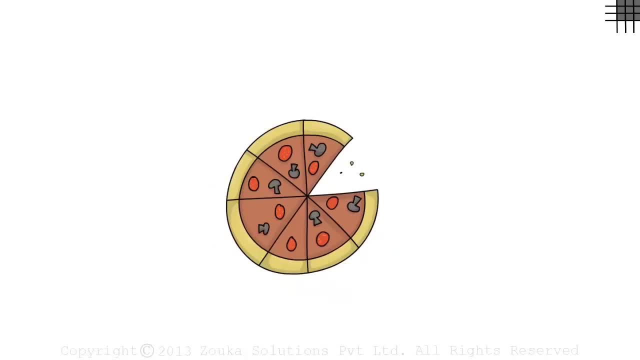 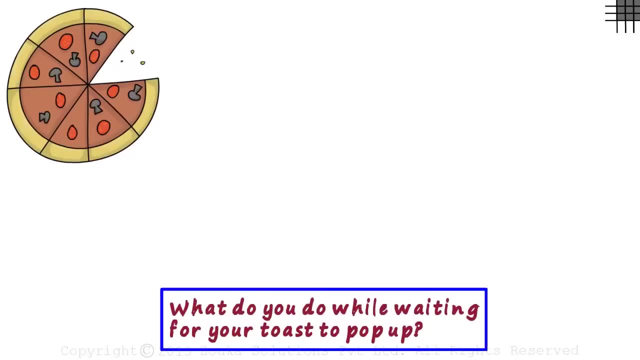 I was looking for some examples of pie charts, But then I thought I should make one myself. So here's the question: What do you do while waiting for your toast to pop up? I drew a circle that represents the number of people I approached. 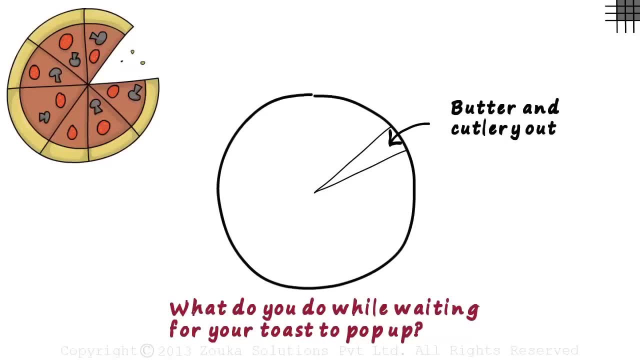 Around 4% of the people told me that they get butter and cutlery out. 2% of the people told me that they clean up the kitchen, And you will not believe that. the remaining 94% told me that they just stare at the toaster. 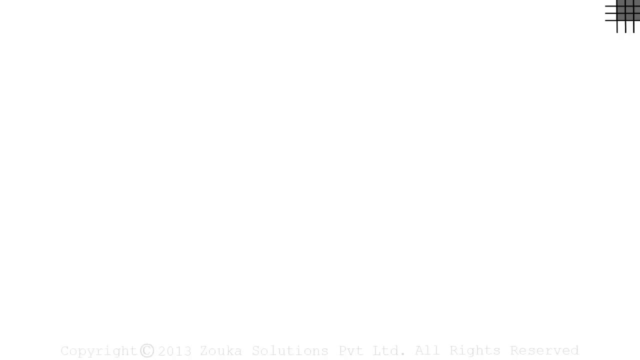 Isn't that true with us too? A few people were asked to categorize the cutlery. They categorized the content of a pop song. A circle was drawn to represent the entire content Around 2% was actual lyrics, 25% was the word yay. 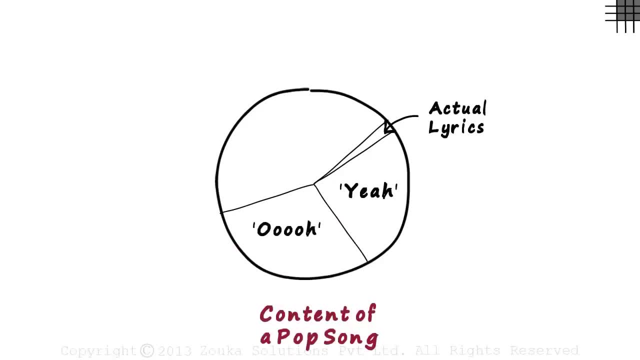 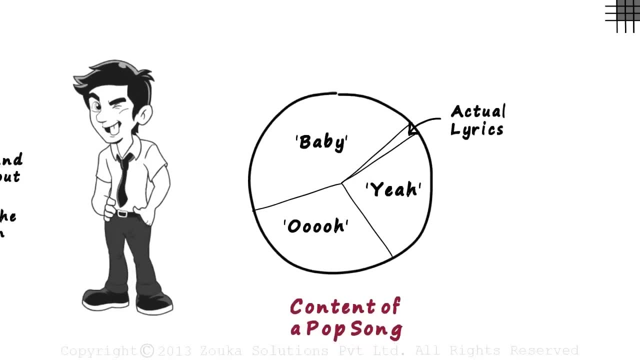 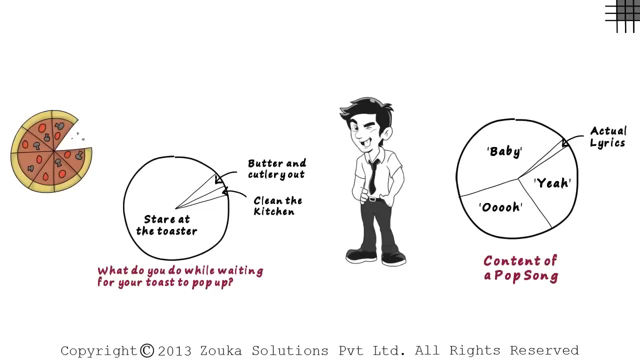 30% was the word ooh And the remaining was the word baby. This was just a funny way to understand pie charts. We will look at a couple of serious examples in our other videos. Thank you for watching.